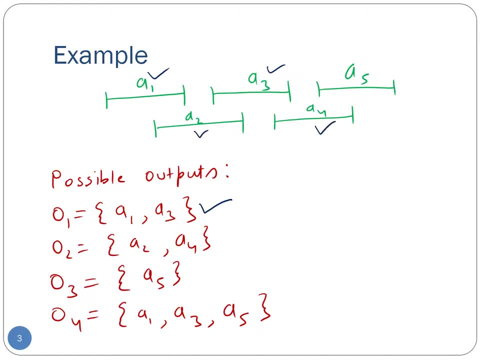 Similarly, a2 and a4 do not have any overlap and therefore a2 and a4 are a possible output subset. any single individual activity, for example a5 itself or a1 itself or a3 itself. it cannot overlap with any other activity because there is only one activity in the subset. so that is also a possible. 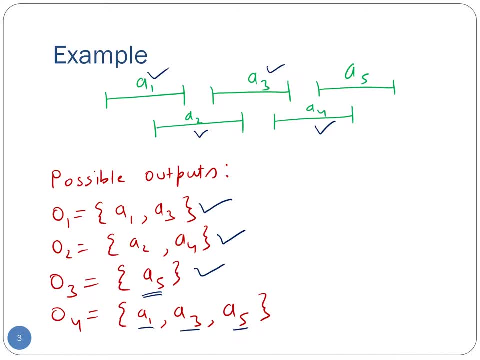 answer similarly: a1, a3 and a5- these three activities here. they do not overlap with each other and therefore this is also a possible output. recall that our goal is to come up with an output subset that has the maximum number of mutually compatible activities. so in this case, 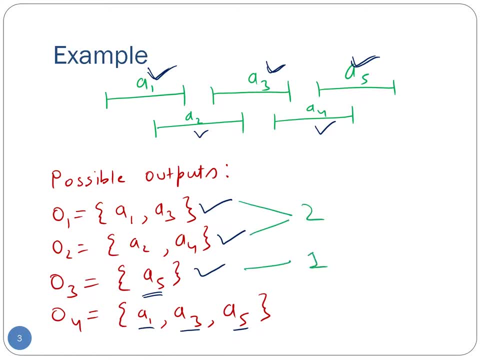 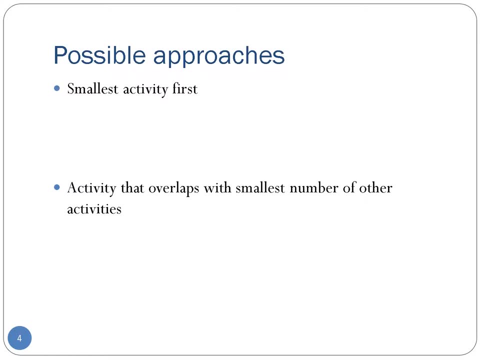 o1 and o2 have two activities, o3 has just one activity and o4 has three activities. therefore, o4 is our optimal answer. let us now try to come up with a greedy algorithm that always computes an optimal solution to this problem. now, because our goal is to select. 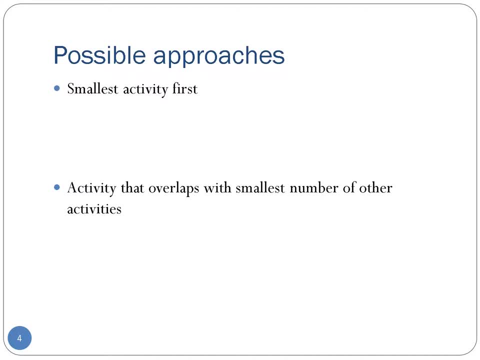 largest number of mutually compatible activities. what if we always select the smallest activity first? would that work? unfortunately, it turns out no, and it is very easy to come up with a counter example. here is one. in this example, a2 is the smallest activity. however, if we first select a2, we cannot select a1 or a3, because a2 overlaps with both. 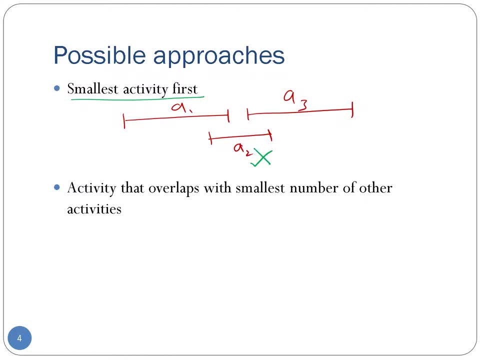 however, that is clearly not the optimal solution. instead of a2, if we selected a1 and a3, we would end up with the larger subset of mutually compatible activities. so what else can we do? what if we always select the activity that overlaps with smallest number of? 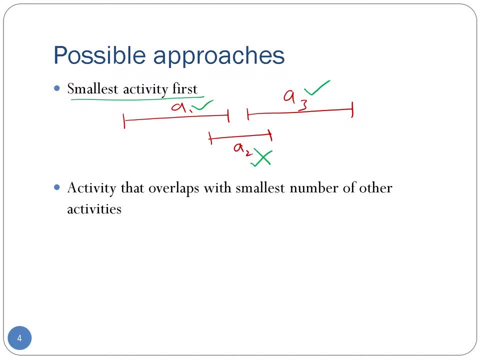 other activities. would that work? maybe not. here is a counter example. in this example activity 6 has overlap with only two other intervals, five and seven. all other intervals have overlap with at least three or four other intervals. so if we pick activity six over here, we cannot pick activity five and activity seven now from. 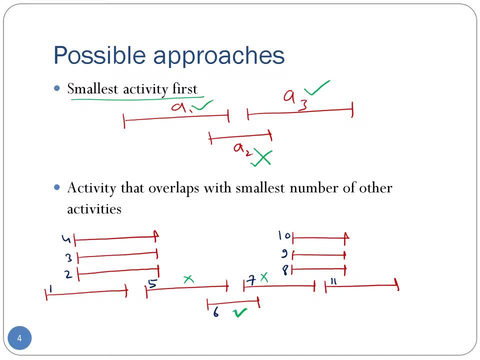 here onwards, no matter which intervals we pick, we can only pick two more. so let us say we pick one and eleven, so we end up with a solution with three intervals, but clearly this is not the optimal solution. we could have instead simply picked interval 1, 5, 7 and 11, and that 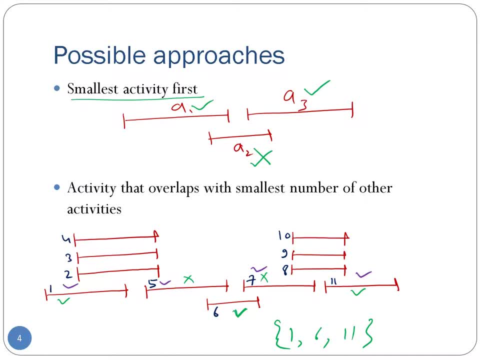 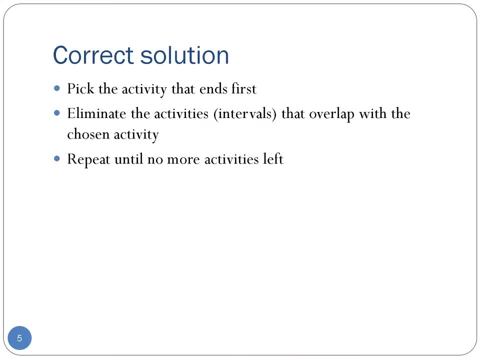 would have given us a mutually compatible subset of four activities, and therefore this is also not an optimal solution. so, likewise, it is easy to come up with several greedy heuristics for solving this problem, and for most of them it is straightforward to come up with counter examples showing they won't work. 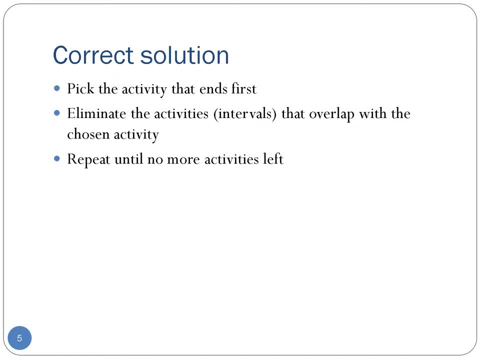 so here is a correct greedy algorithm for the problem that always works. so first we sort the input set of activities in increasing order of their finish times, then we pick the activity that ends first. after this we eliminate all those activities that have an overlap with the chosen. 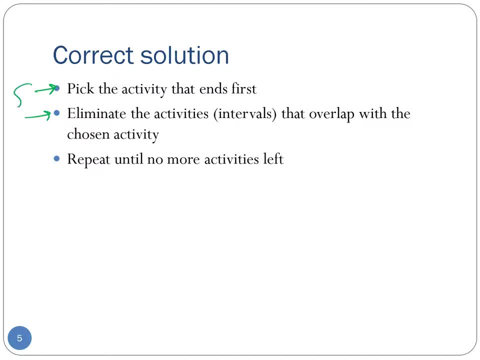 activity, and after this we simply repeat the first two steps on all the remaining activities until there are no more activities left. so here is an example to illustrate the working of this algorithm. so of all these activities, activity one is the one that ends first. all other activities: 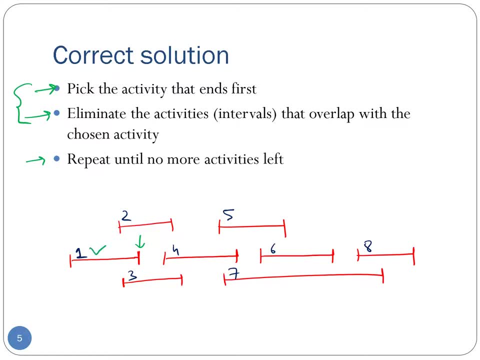 are ending after this point, so we select ned activity 1.. Having done that, we need to throw away those activities that have an overlap with activity 1.. So clearly, activity 2 and activity 3, which overlap with 1, they cannot be in our. 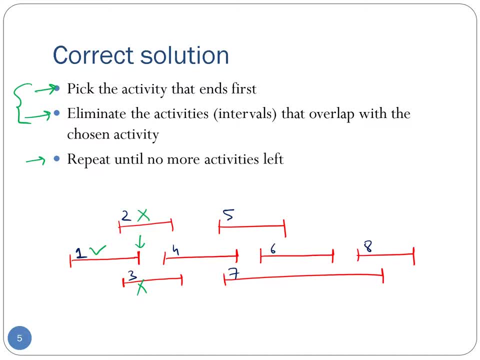 solution. Now we simply repeat this on the remaining activities. So activity 4 is the one that ends next. All other activities are ending after this point. So we next choose activity 4 and we have to throw away the overlapping activities with 4.. So activity 5 and activity 7. 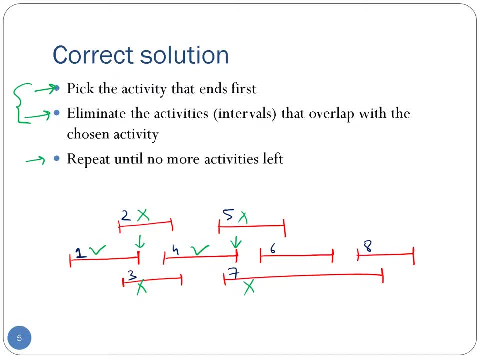 that overlap, they cannot be part of the solution. After this, activity 6 is the next that ends. So we choose activity 6, and if there are any other remaining activities that overlap with 6, they need to be thrown away. but there are no such activities right now. The only other remaining. 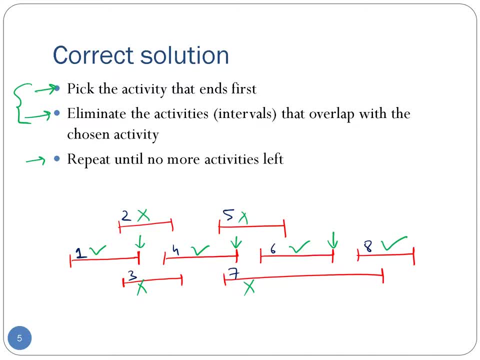 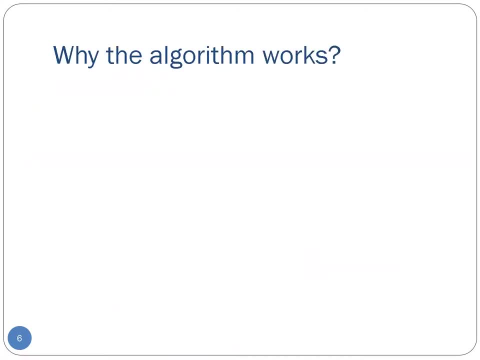 activity is activity 8, which has no overlap with the chosen activities. So this is our final answer. activity 1,, 4,, 6 and 8 is the final answer. So why this algorithm works. A detailed proof of correctness is beyond the scope of this video, but here is an insight that 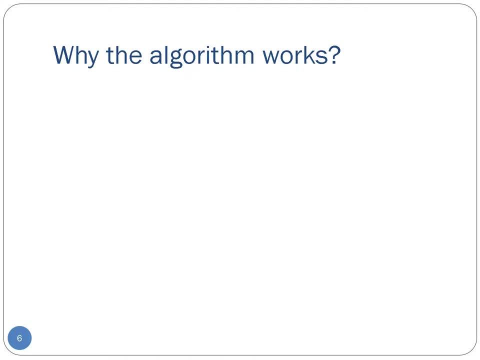 will help you appreciate the algorithm. Any correct solution to the problem would look something like this: Essentially, a series of activities that do not overlap To this solution. if you add an activity that ends first, assuming it is not already part of the solution, one of two. 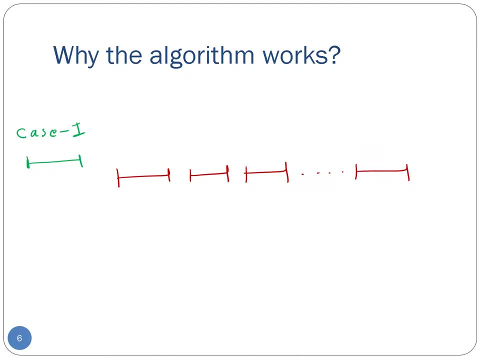 things would happen. In the first case, if the activity that ends first does not overlap with the first activity of your solution, adding it will improve your solution. Another possibility is the activity that ends first has an overlap with the first activity of your solution. So, adding the interval that ends first, you will have to drop the first interval or first activity. 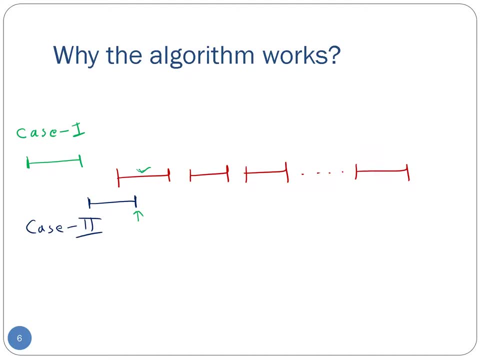 of your original solution, But note that the overall size of your solution remains the same. You dropped one interval and you added one interval. Therefore, adding the interval which gives you the desired length would be the same as adding another interval. However, the activity that ends first can not make your solution any worse. It can only. 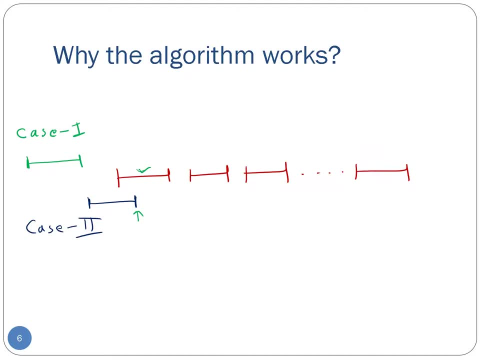 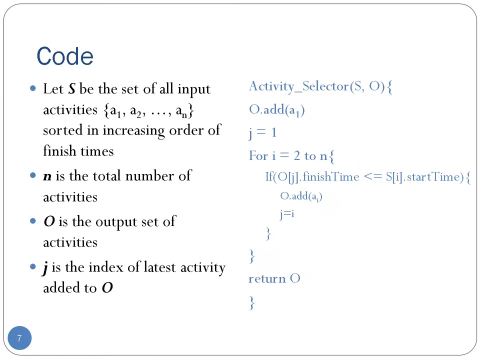 improve it. Also, note that the activity that ends first cannot have an overlap with more than one activities in your original solution. Since it is the activity that ends first, it must end before or at the same time as the first activity of your original solution. 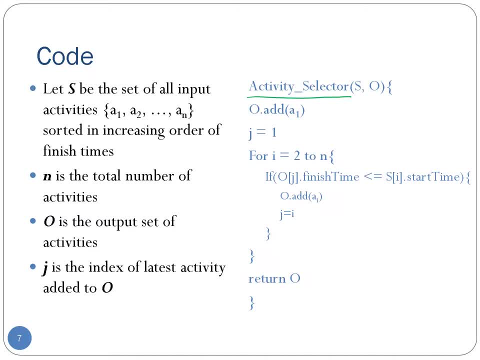 iterative function for solving the activity selection problem. capital s is the input set of all the activities, a1, all the way up to a n. we assume that activities are sorted in increasing order of finish times, so a1 finishes before a2, and so forth up to a n. 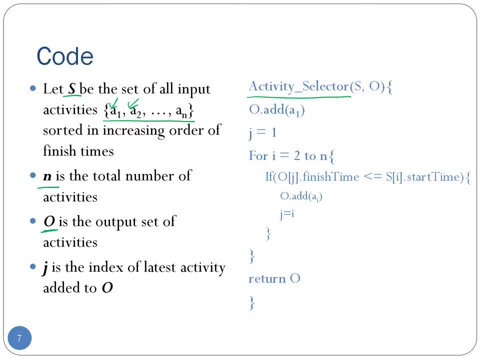 the total number of activities is n. capital o is the output set, the desired output set of activities that are all mutually compatible, and j is the index of the latest activity that is added to capital o, the sub the output set. the output set o is initially empty, so as the function begins execution in the 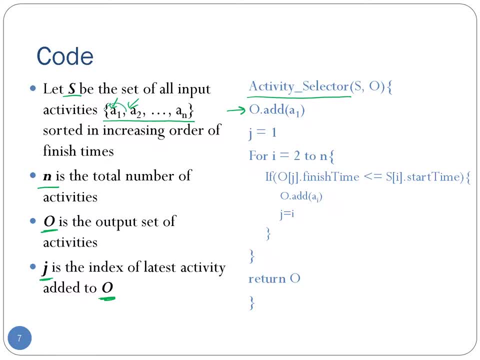 first line. we can directly add activity a1, the first activity in set s, to set o, because recall that these activities in set s are sorted in increasing order of finish times. and then we said: j is the index of all the activities, a1 all the way up to a n.